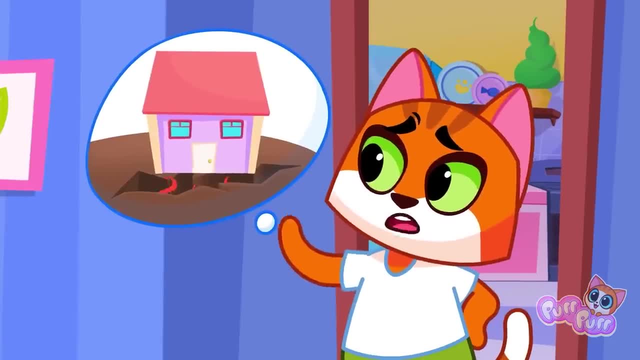 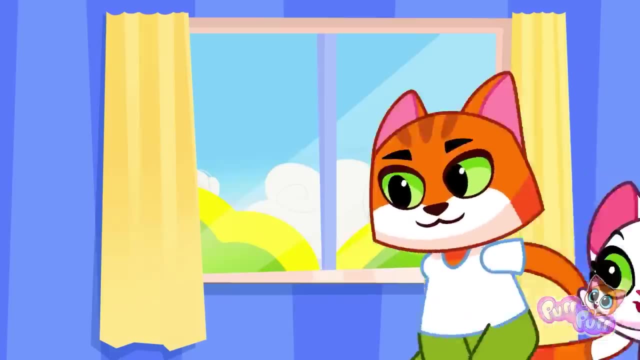 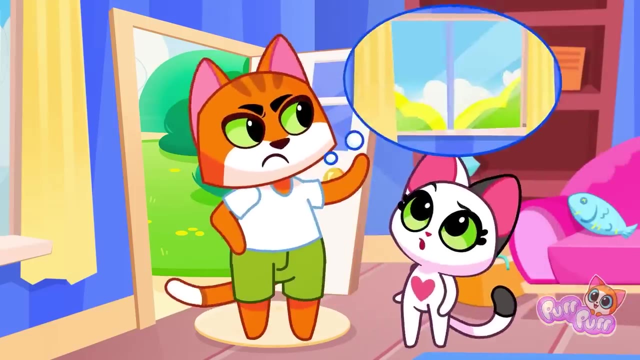 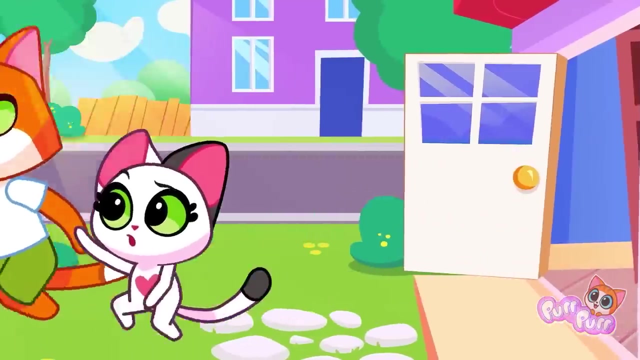 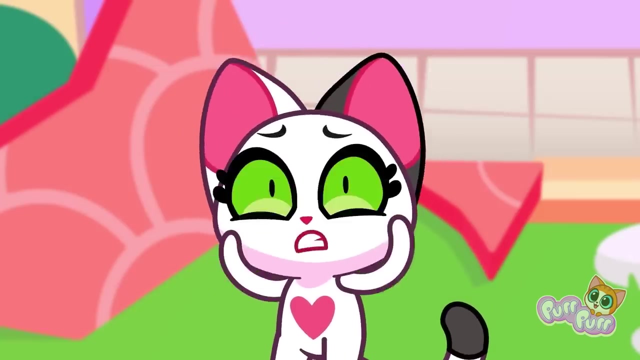 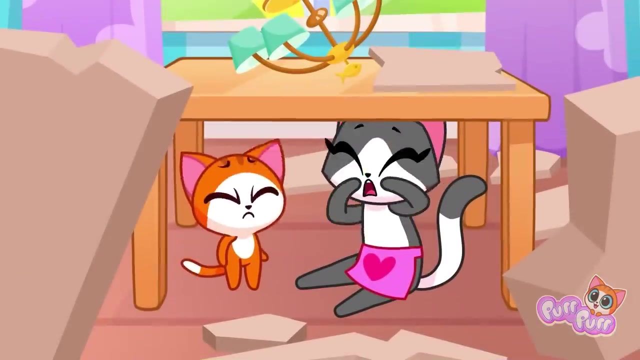 It's all over. We should get out of the house. It can be ruined by aftershocks. Do not approach glass objects. Oh no, We're a mummy and Leo Help us. The rescue team should hear. Hear us. 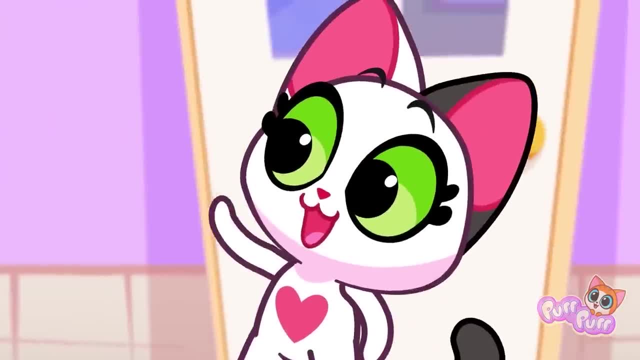 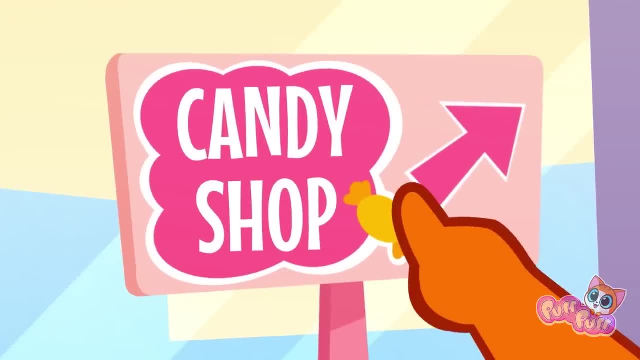 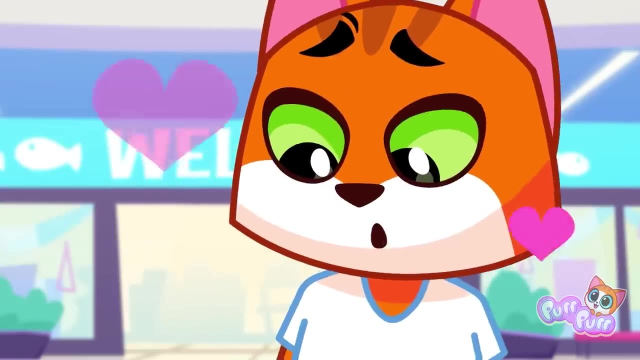 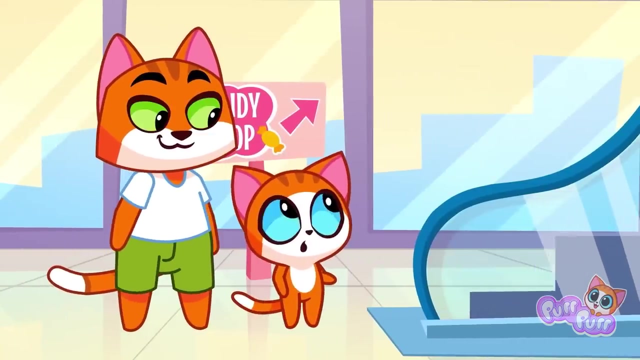 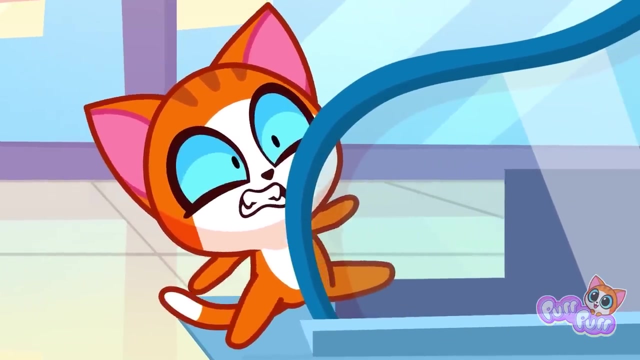 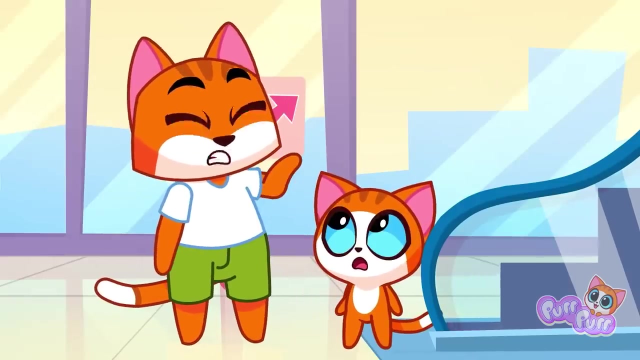 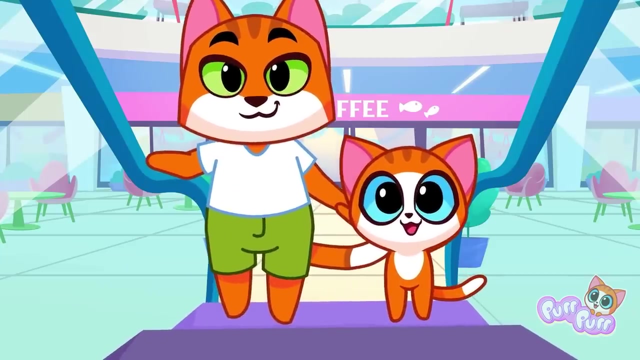 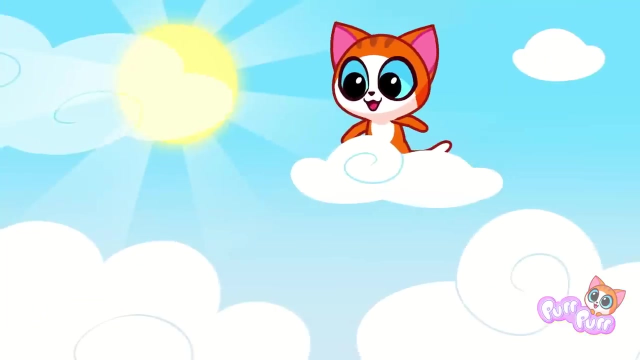 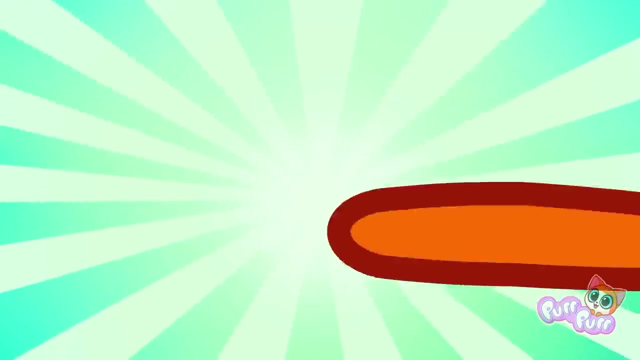 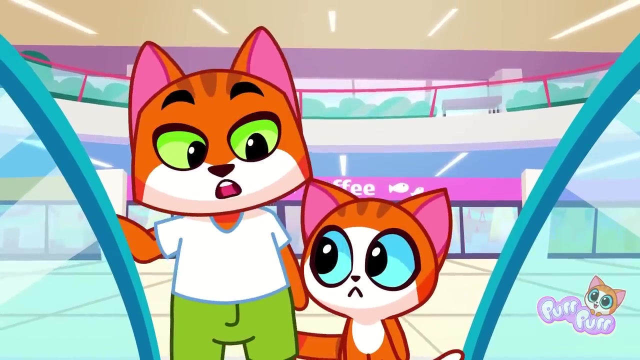 Win the game. Thank you, Cheers. Here's to the next time the baby is baby-ing this book. The baby is baby-ing this book. Leo, the escalator is always moving. When using the escalator, always hold the handrail. 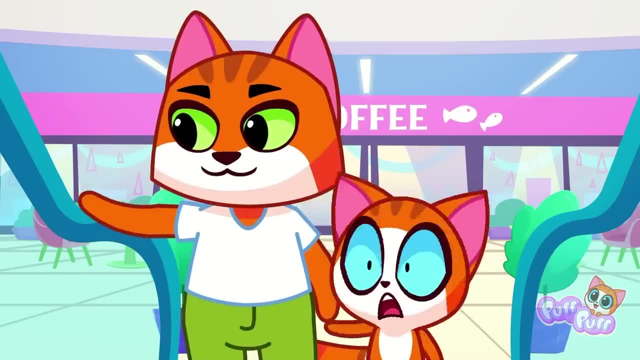 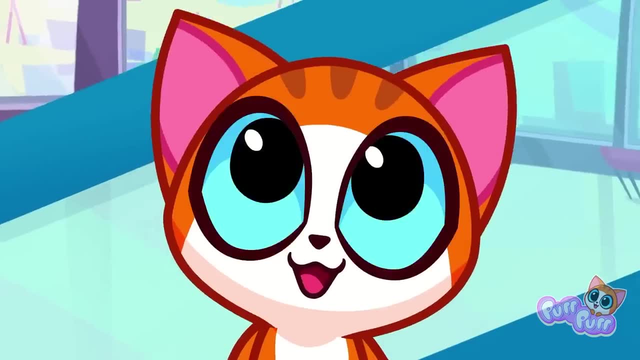 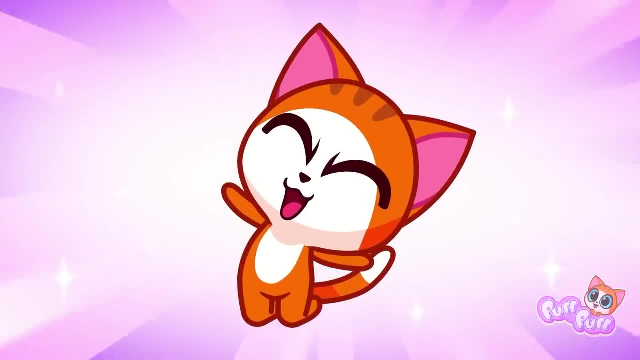 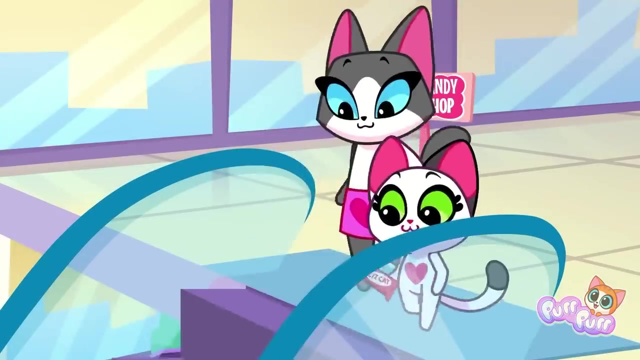 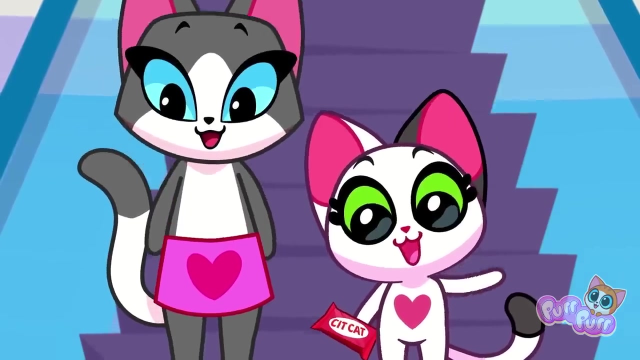 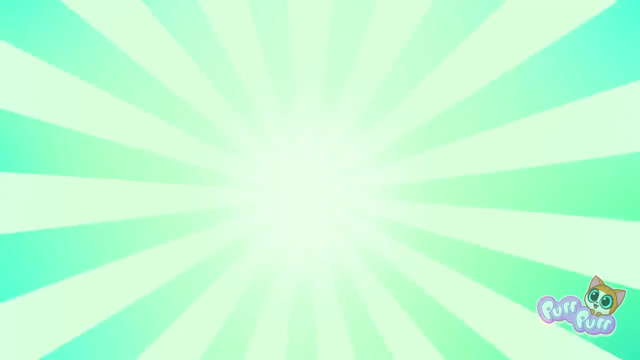 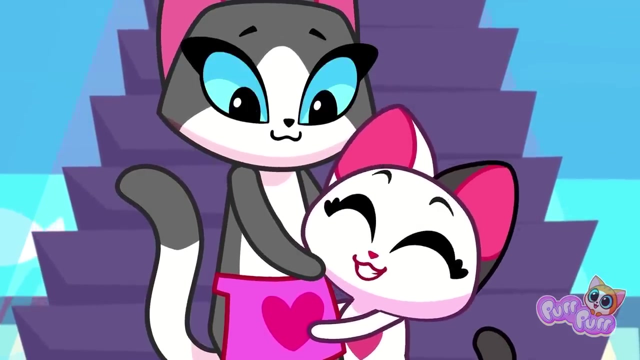 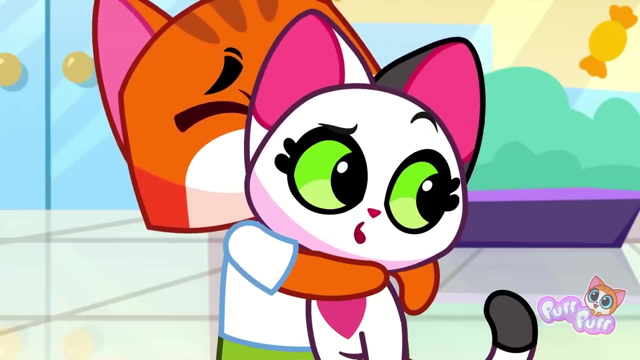 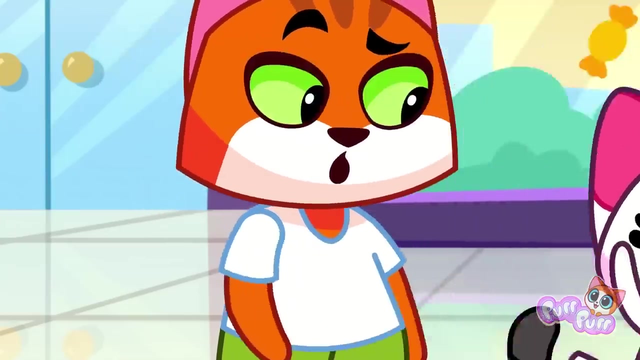 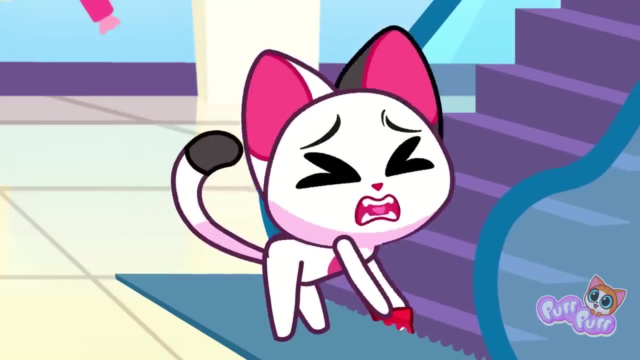 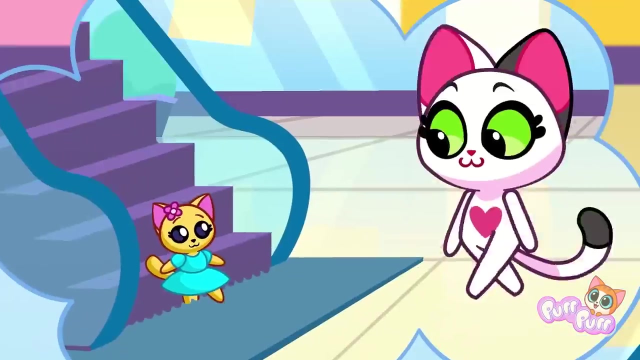 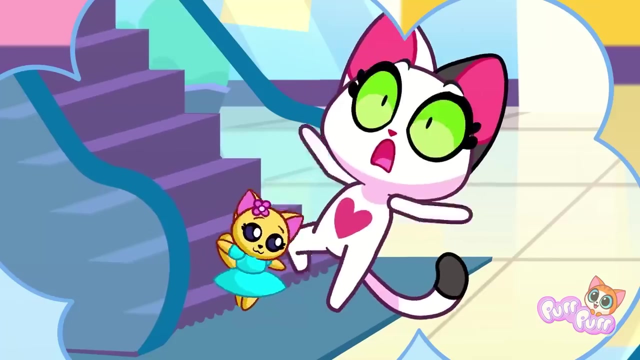 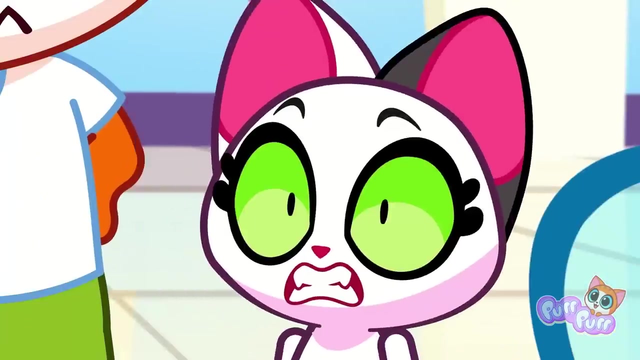 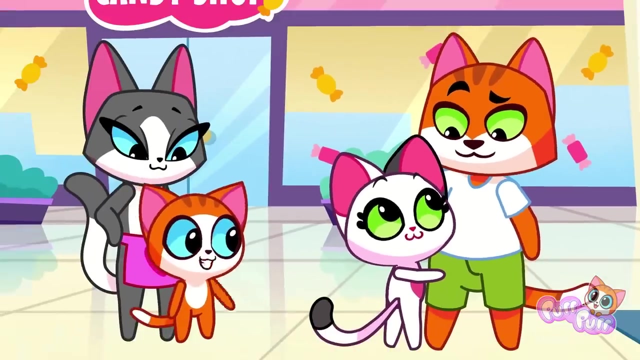 Now you should just step forward, Daddy Leo, Lucy, never run on the escalator. Lucy, be careful, you can get stuck What? I will always be careful on the escalator, Me too. Meow, Meow. 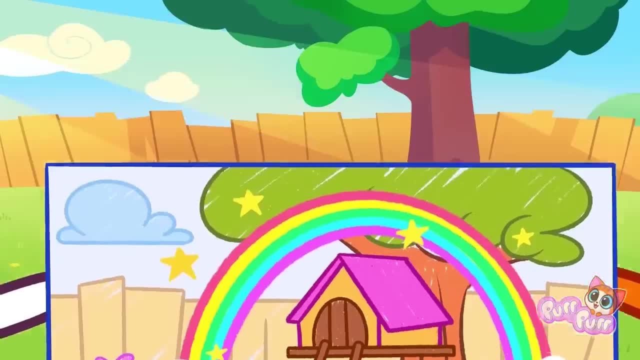 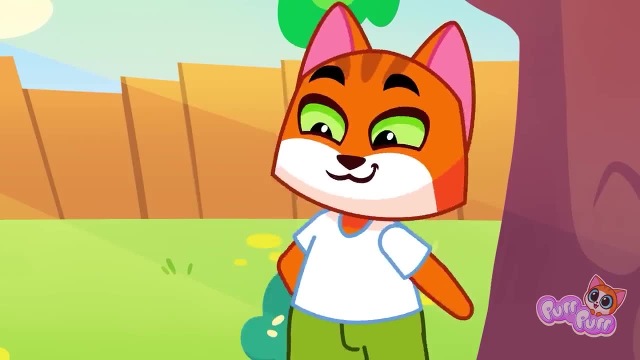 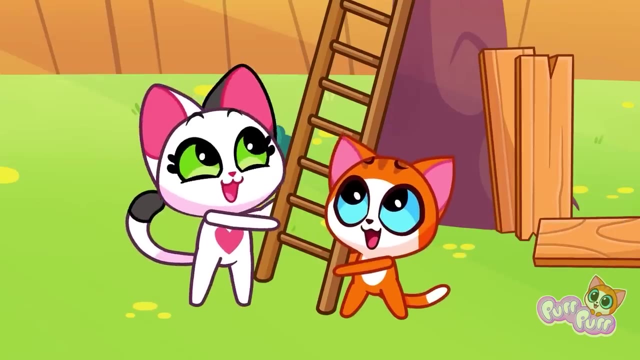 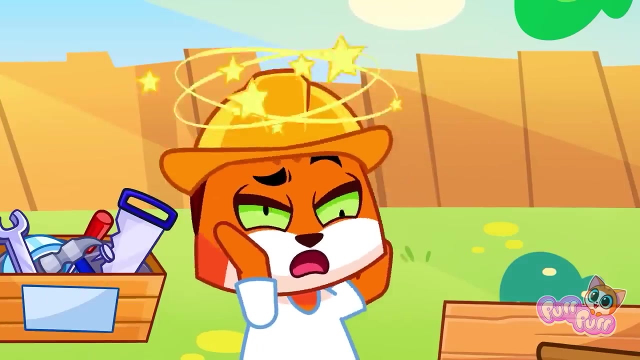 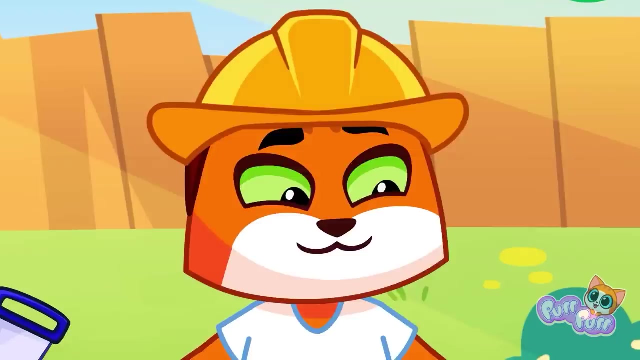 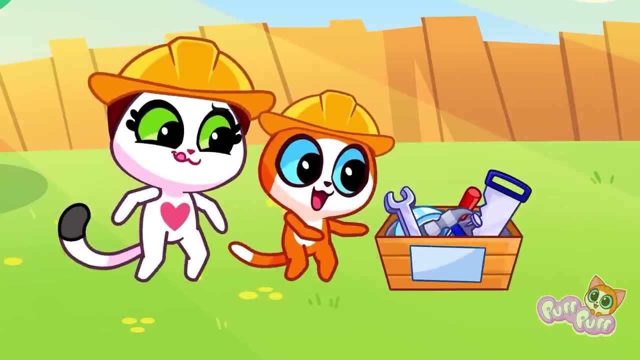 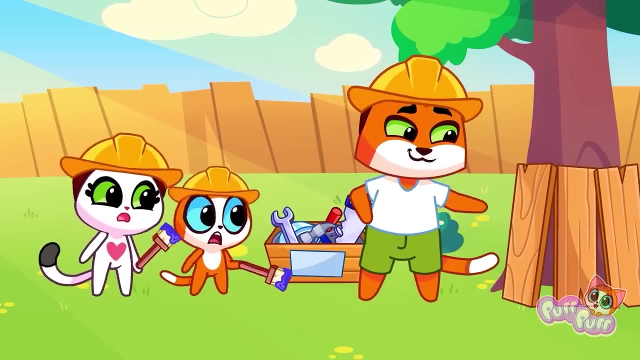 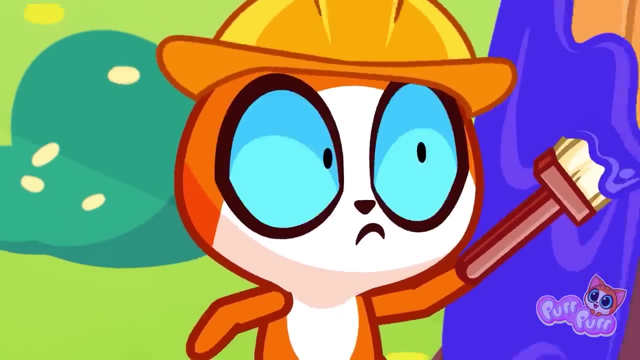 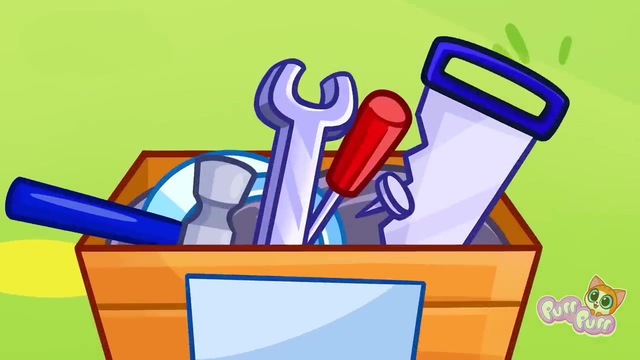 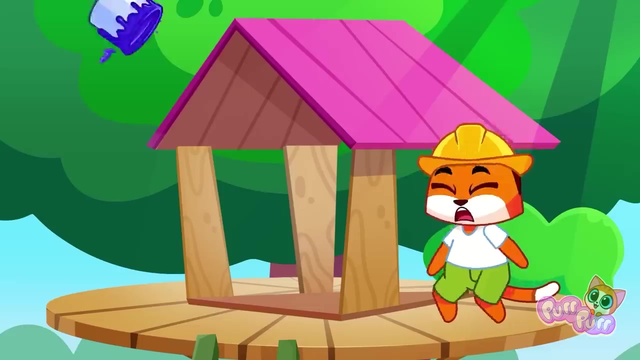 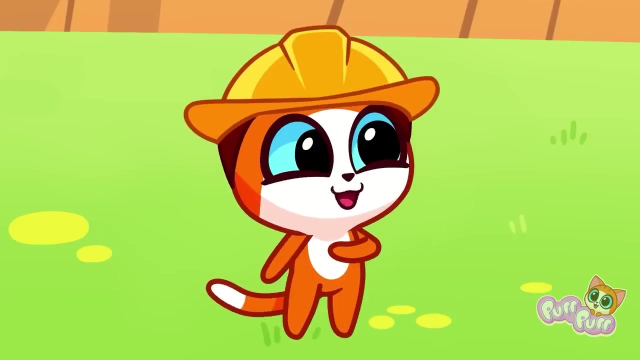 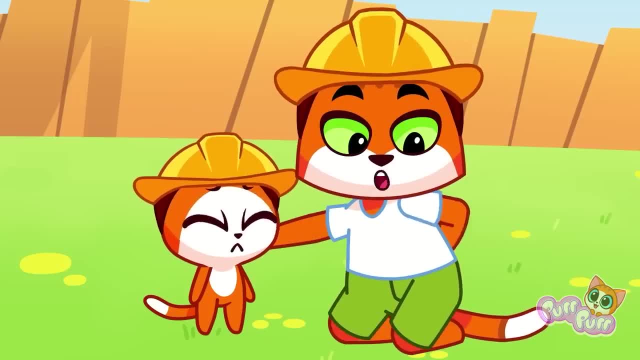 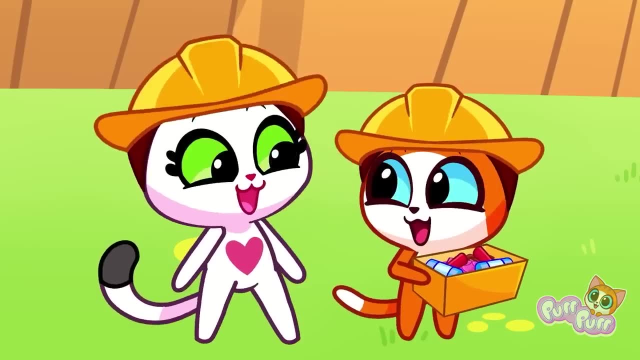 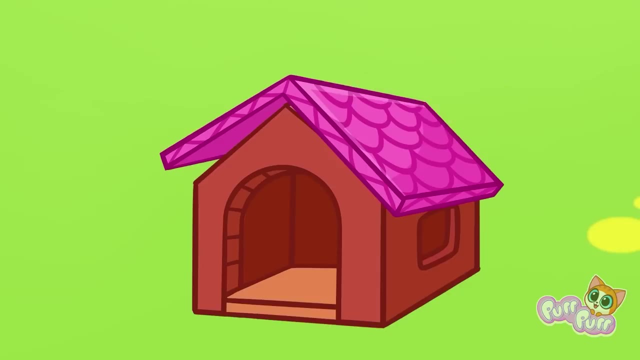 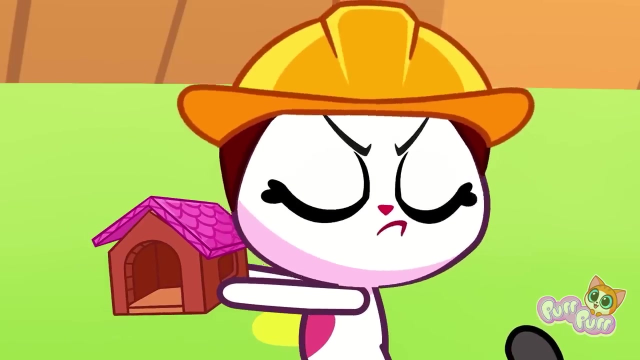 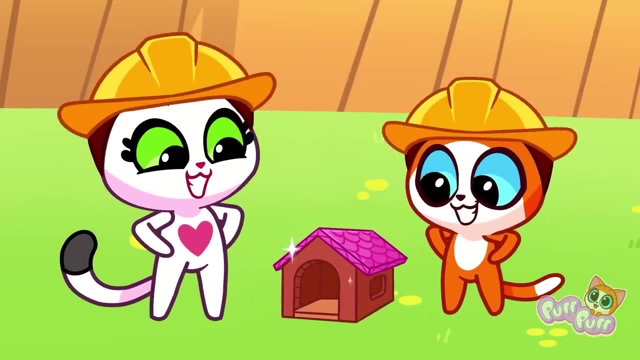 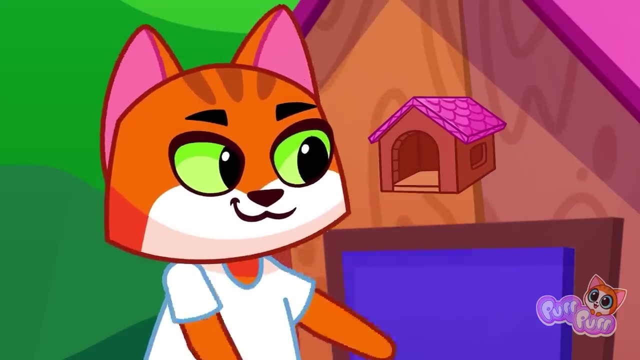 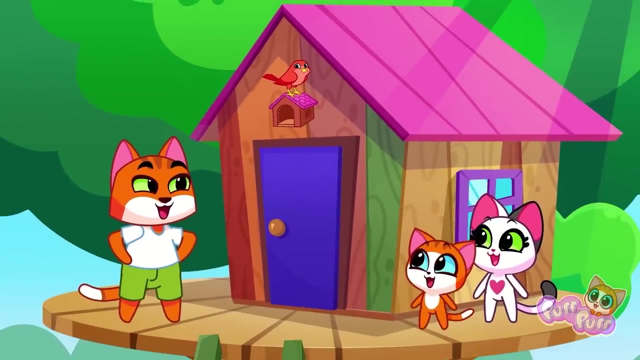 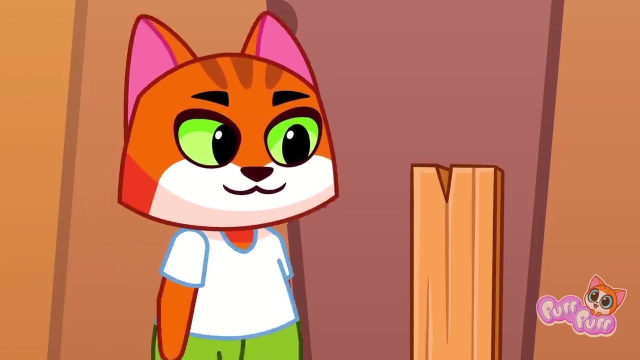 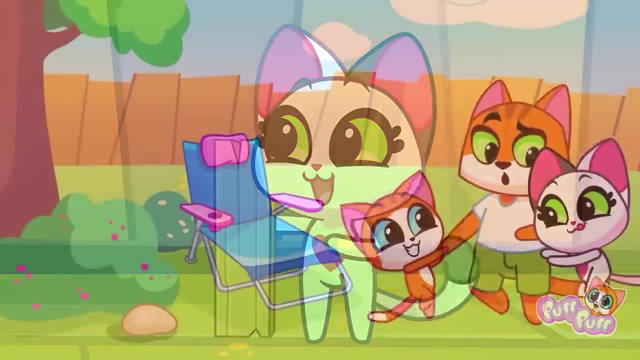 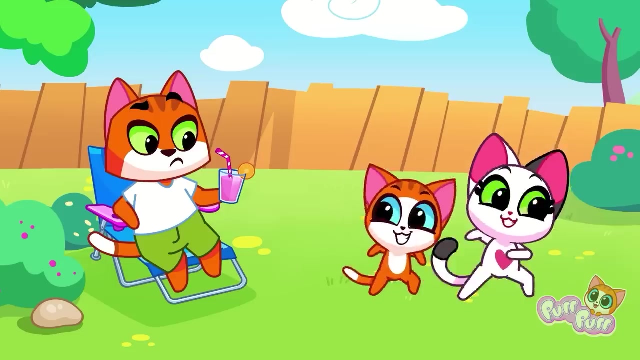 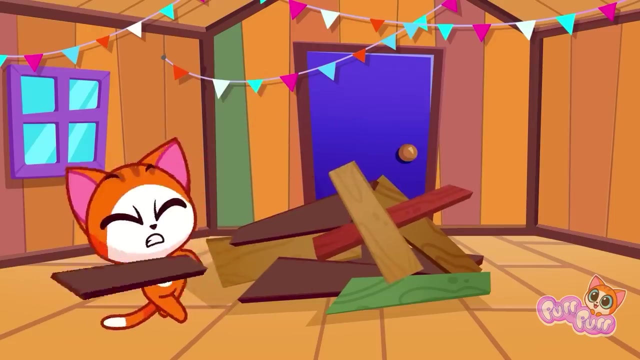 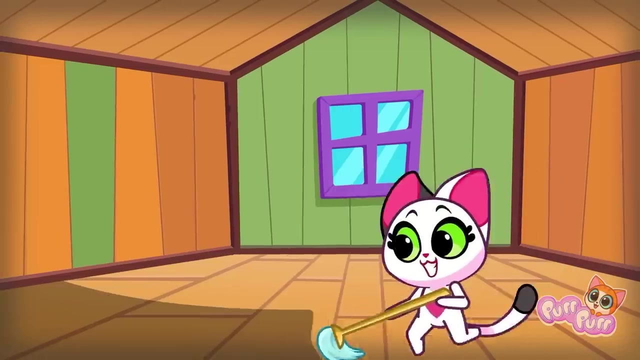 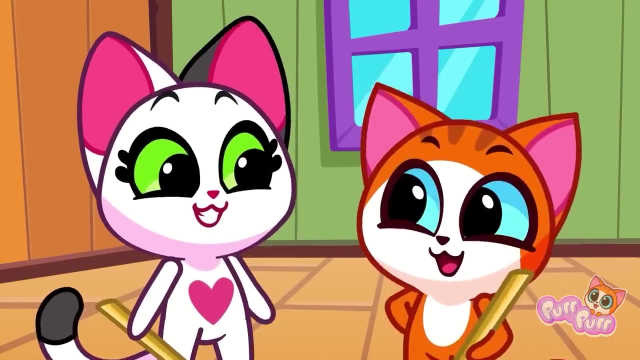 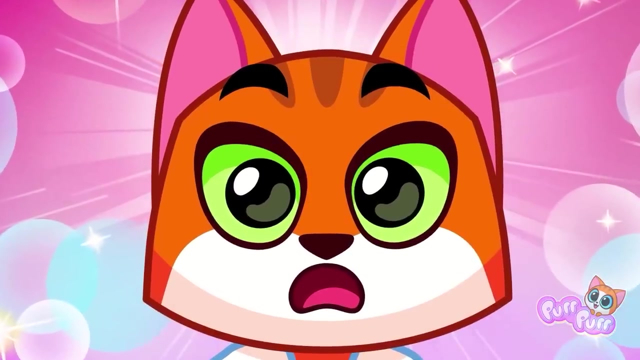 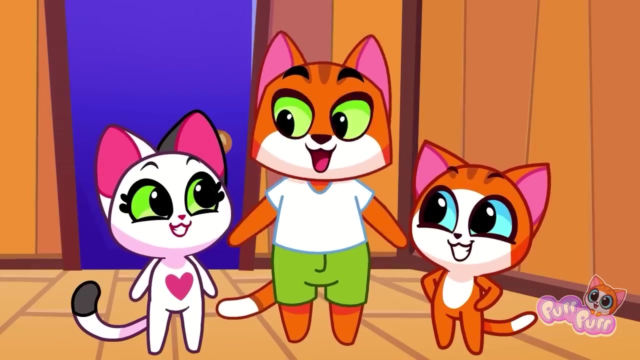 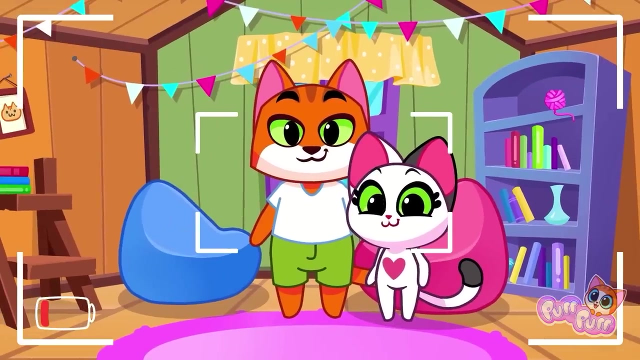 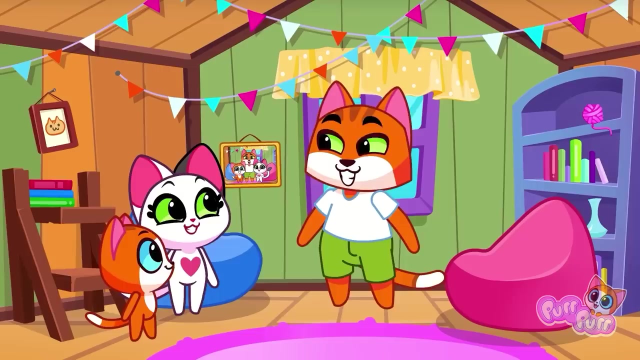 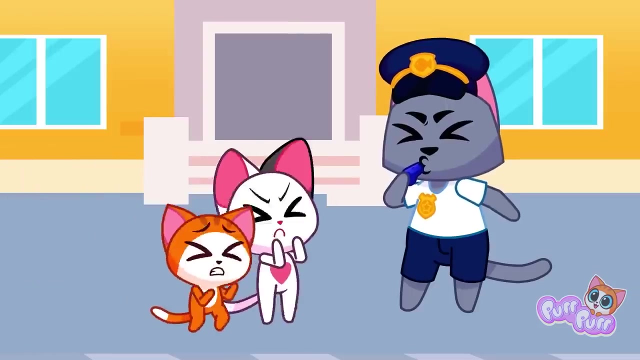 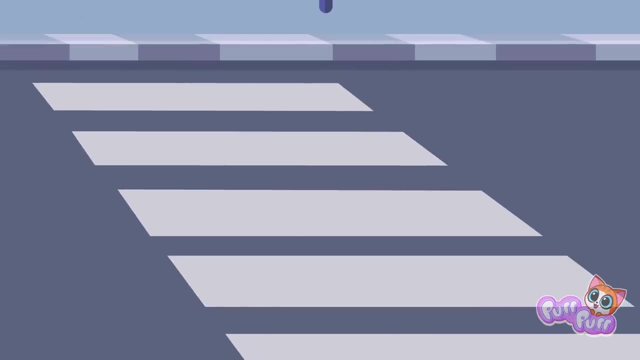 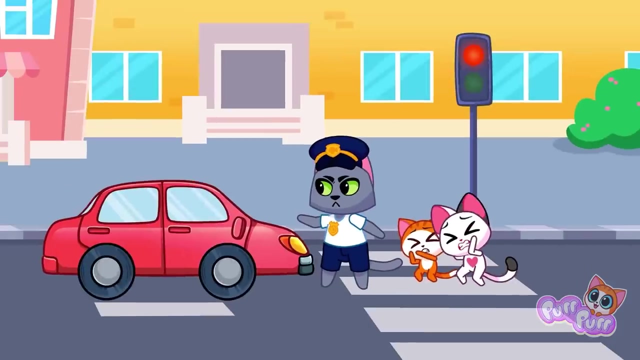 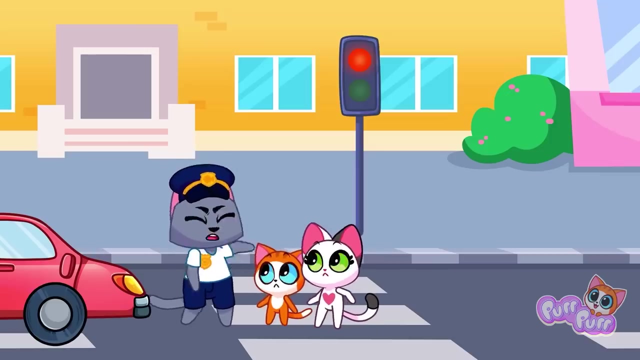 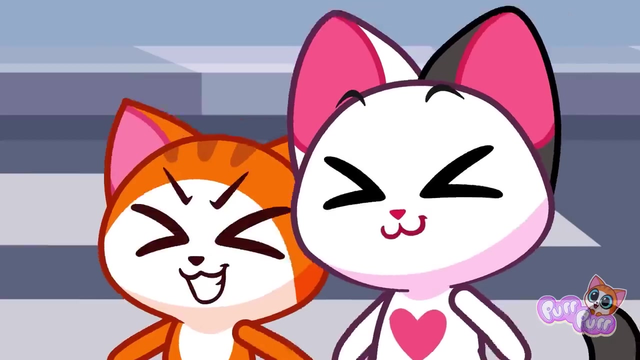 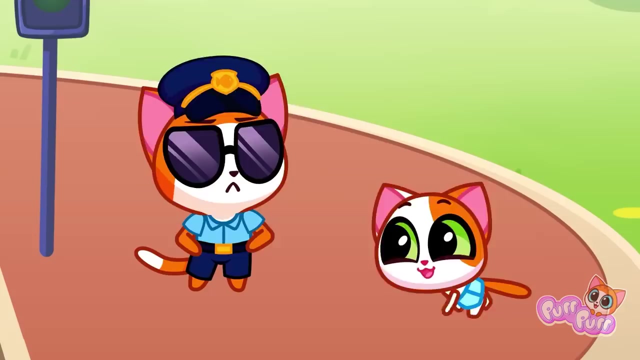 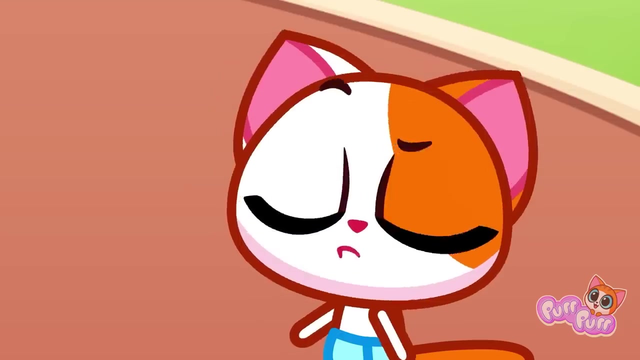 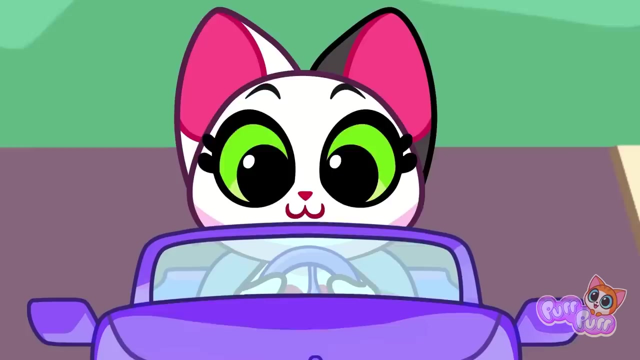 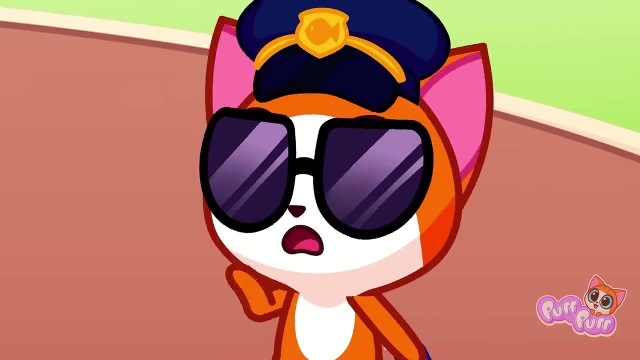 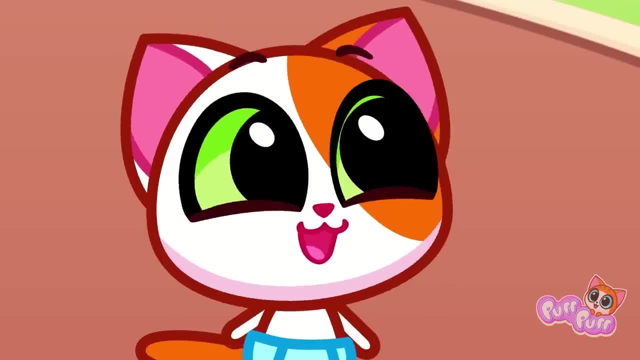 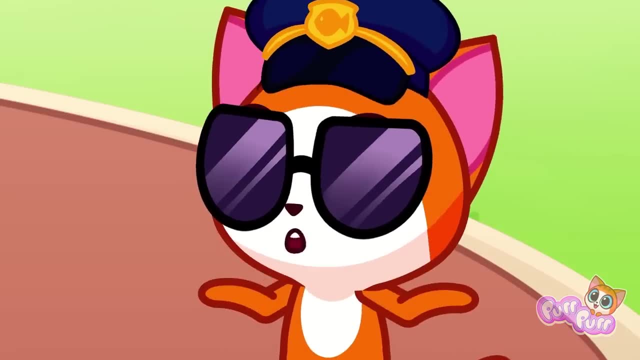 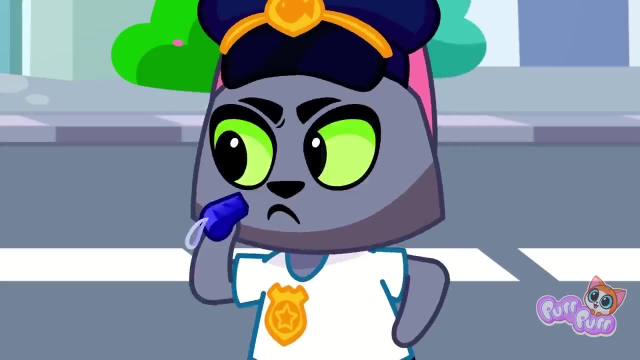 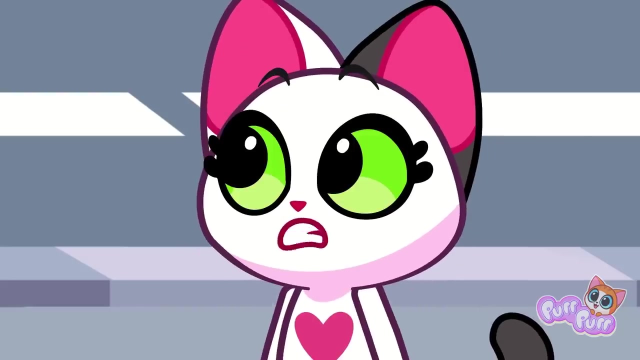 I want to build a treehouse. Green light go. The green light is broken. What shall we do? How to cross the road when the traffic light is not working? How to cross the road when the traffic light is not working? In this case, look at the traffic controller. 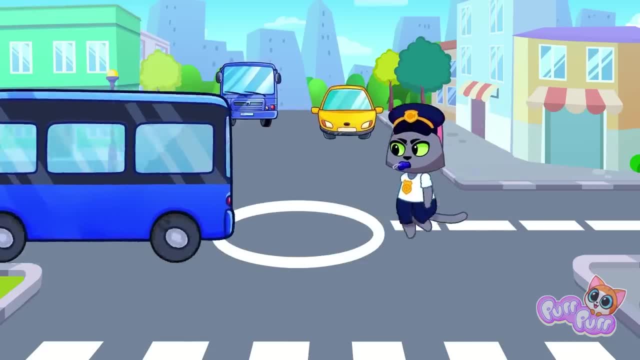 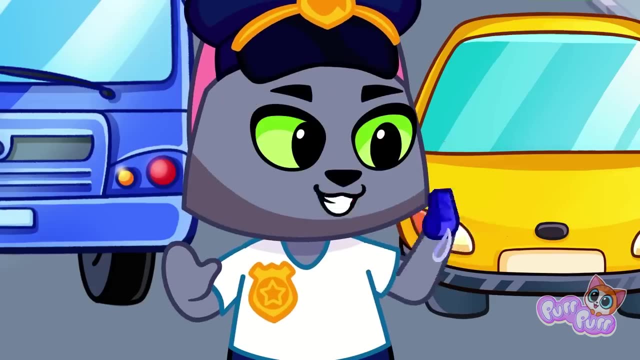 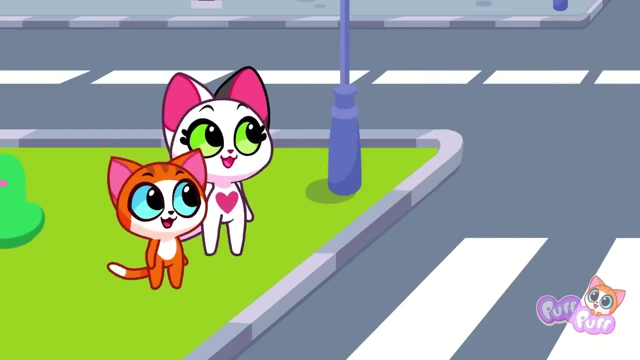 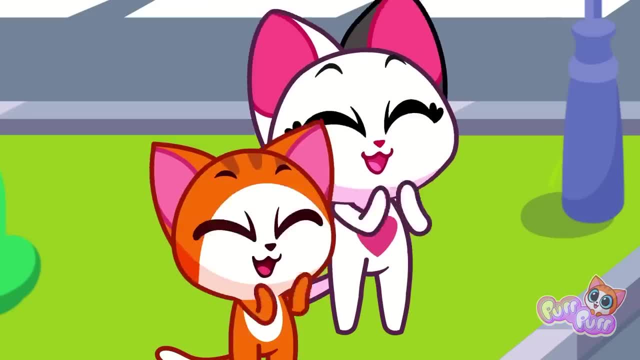 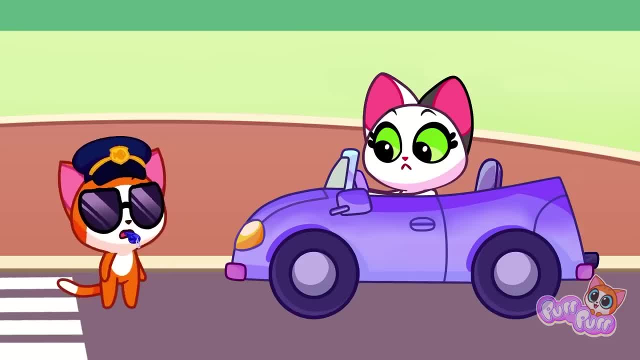 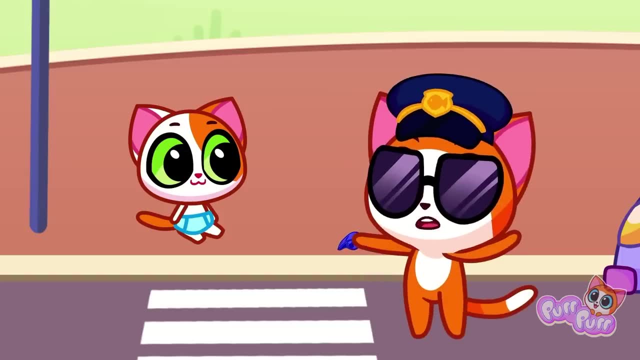 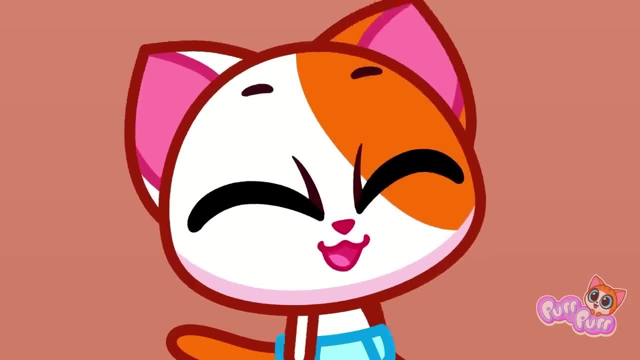 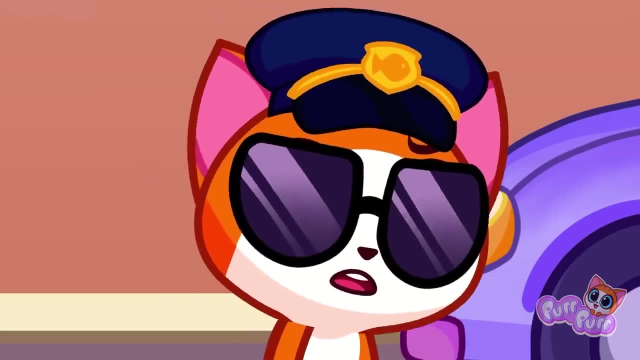 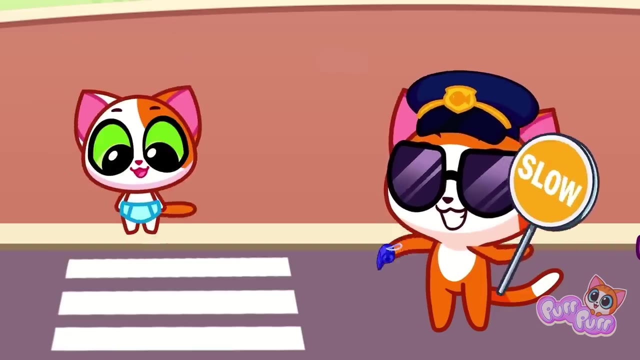 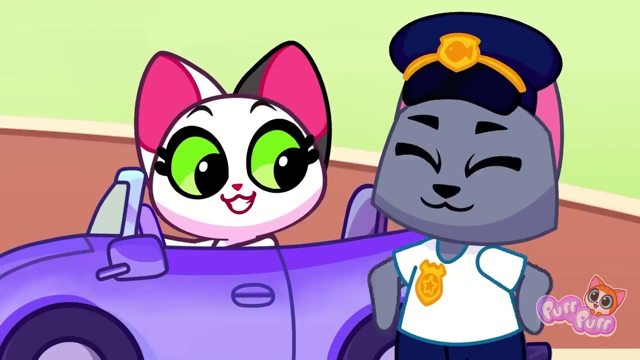 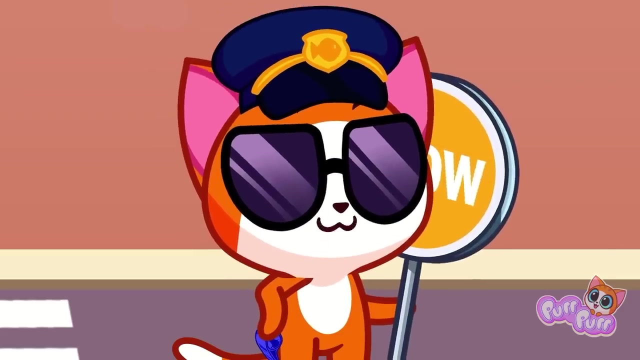 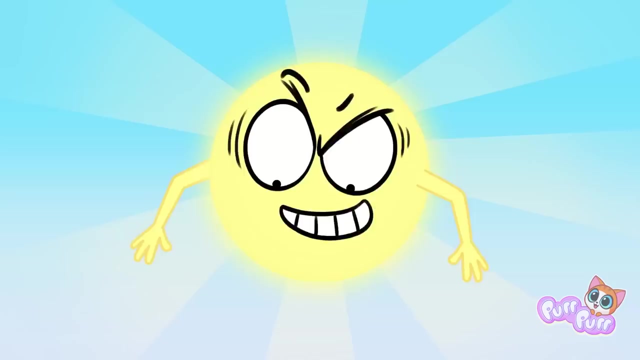 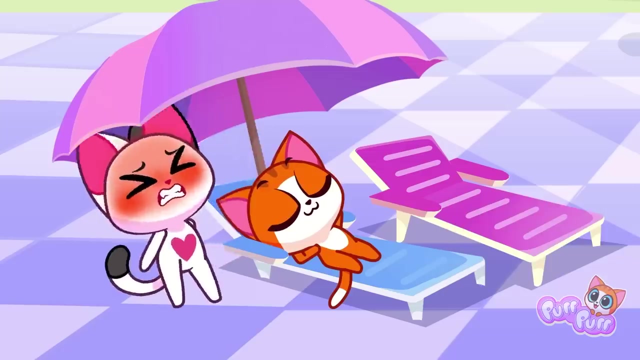 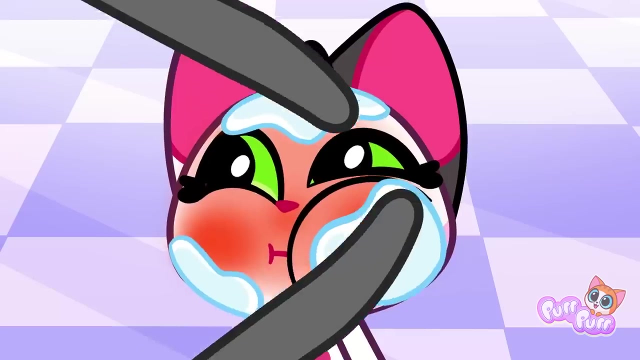 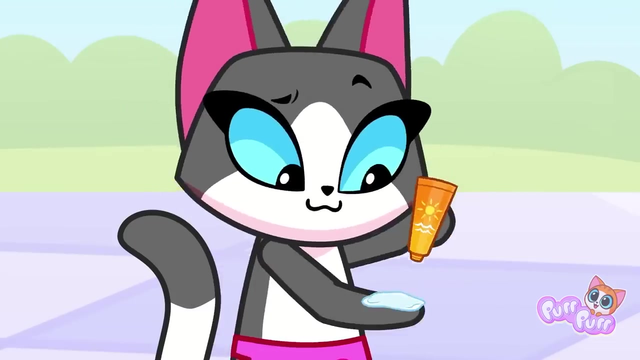 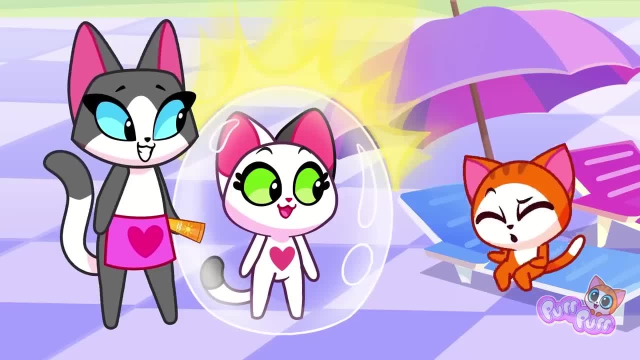 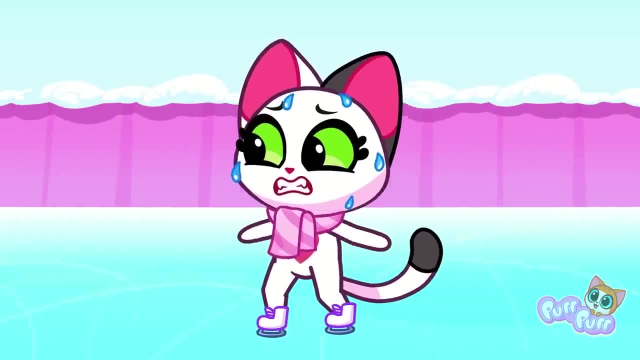 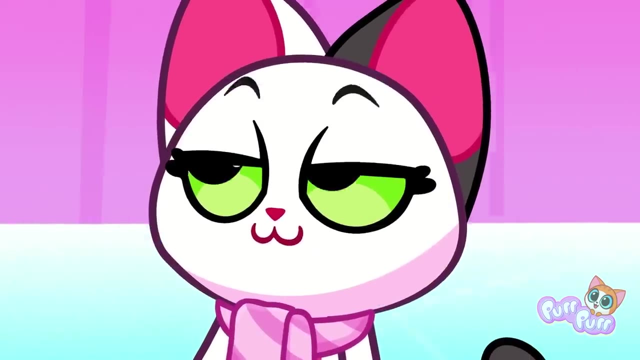 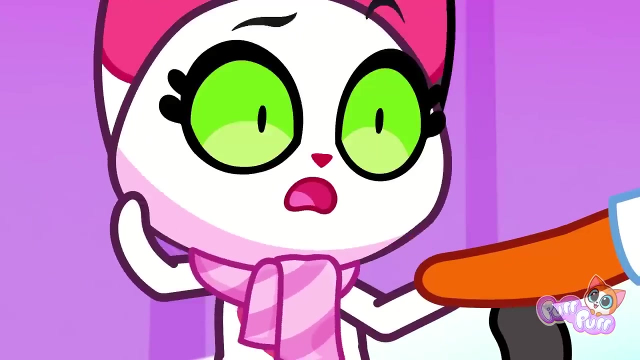 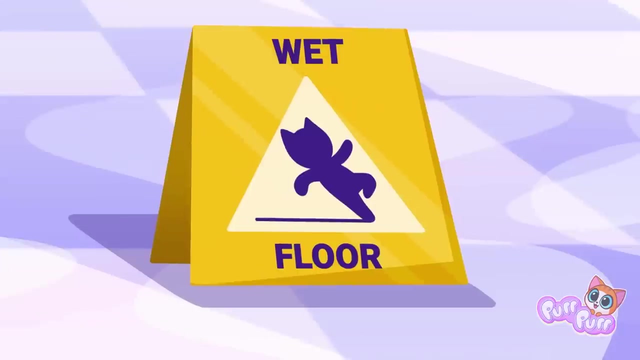 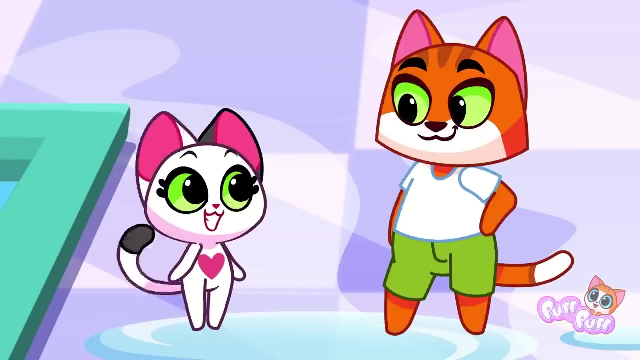 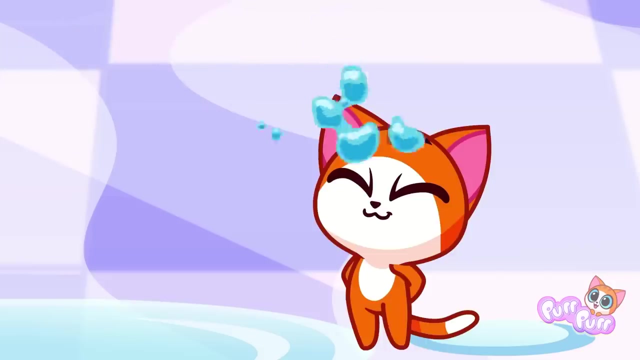 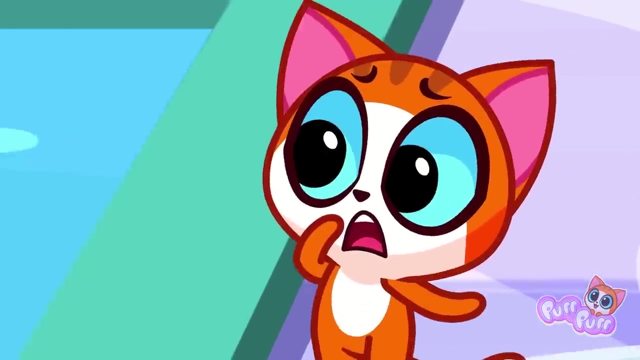 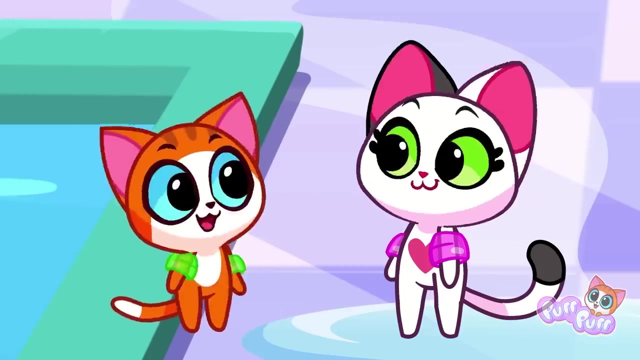 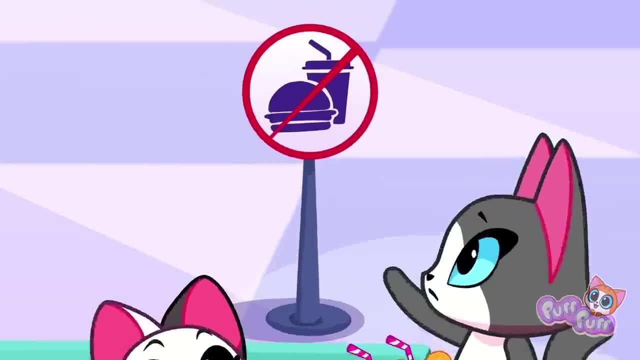 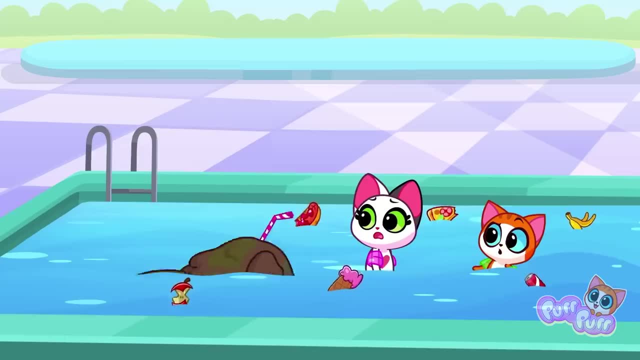 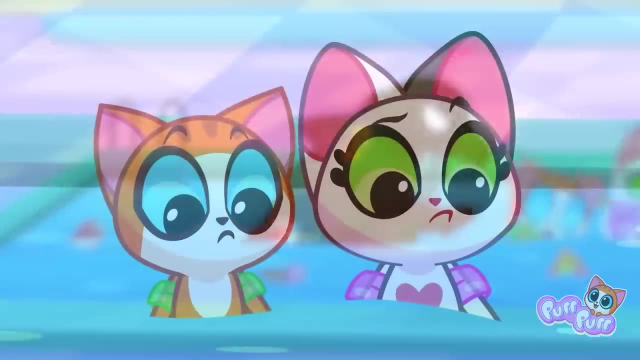 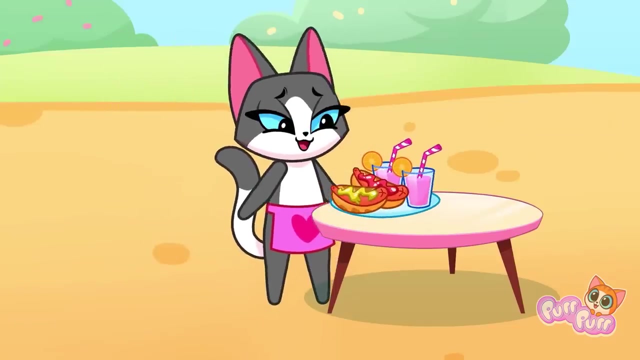 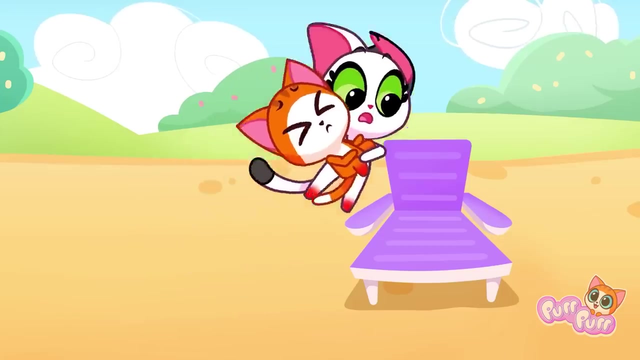 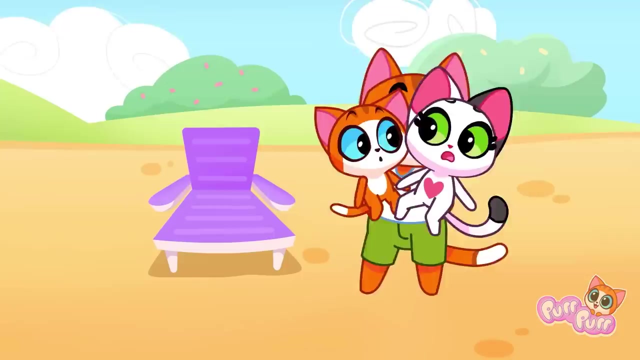 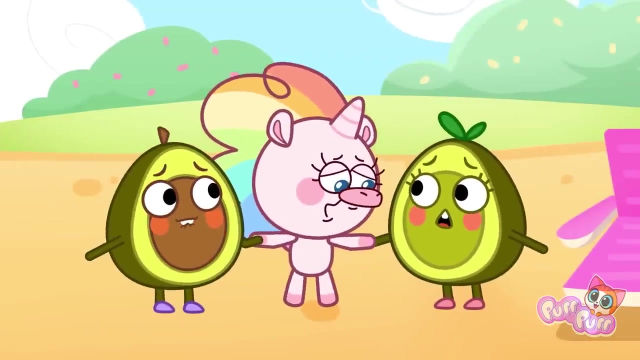 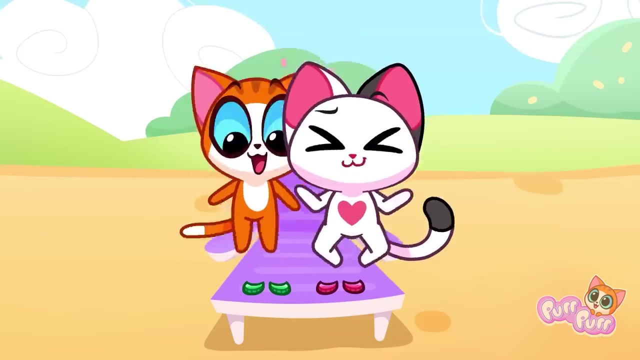 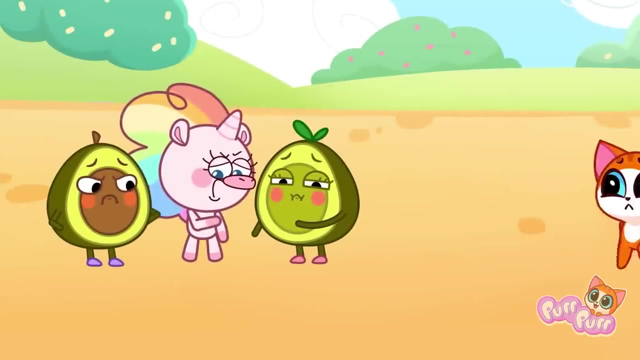 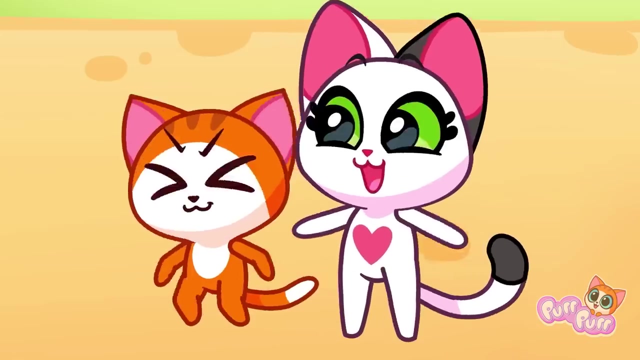 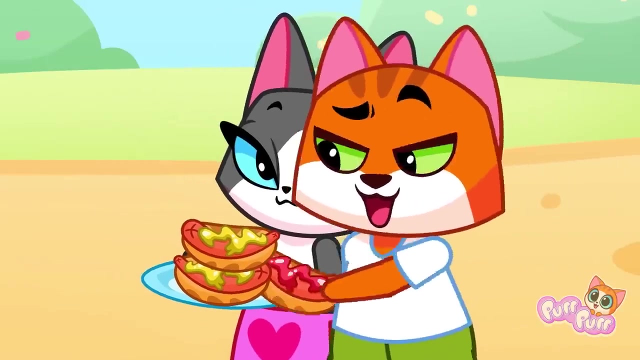 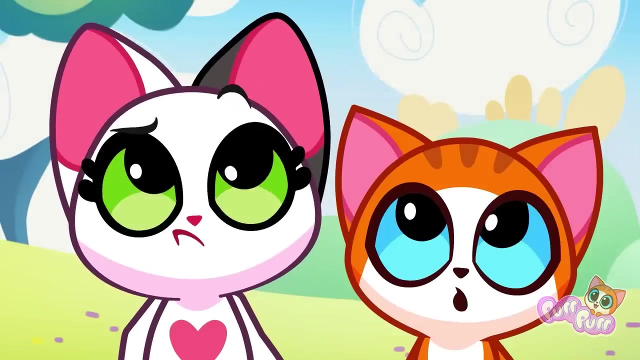 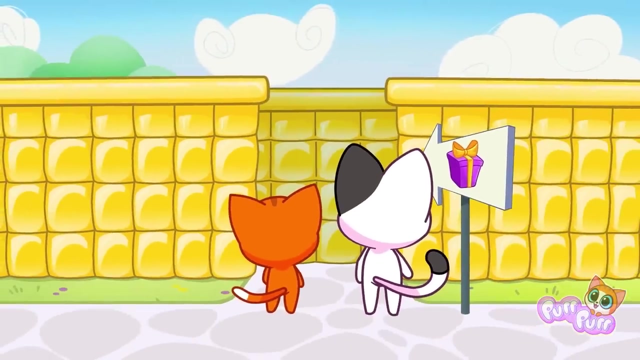 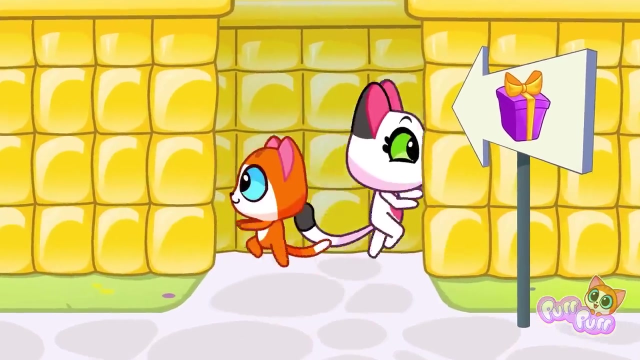 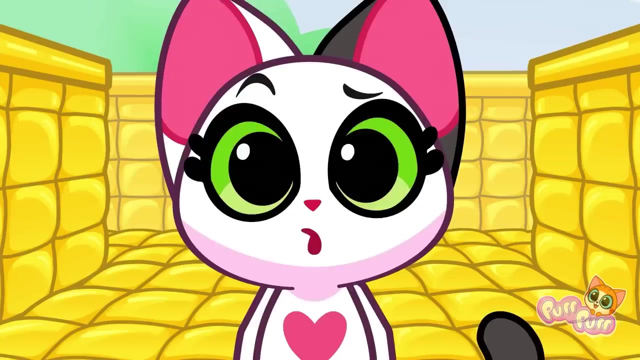 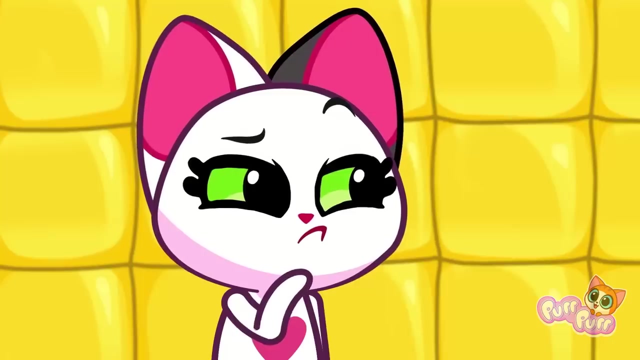 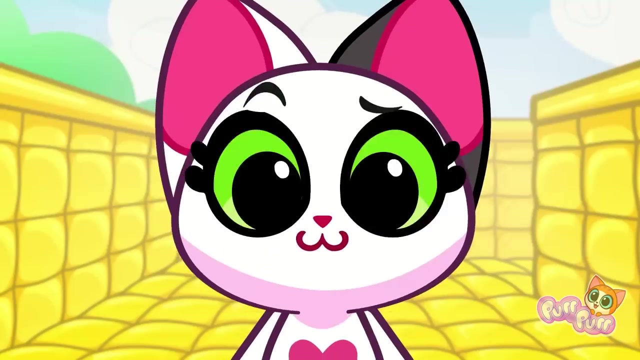 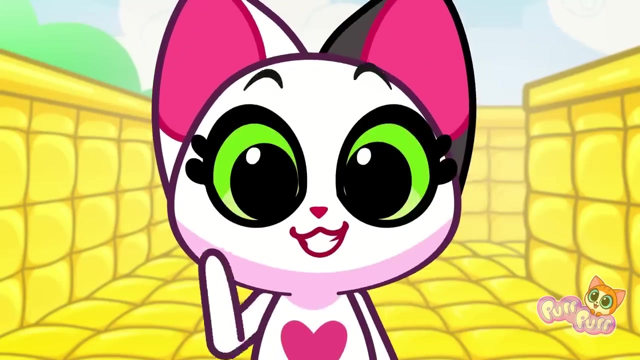 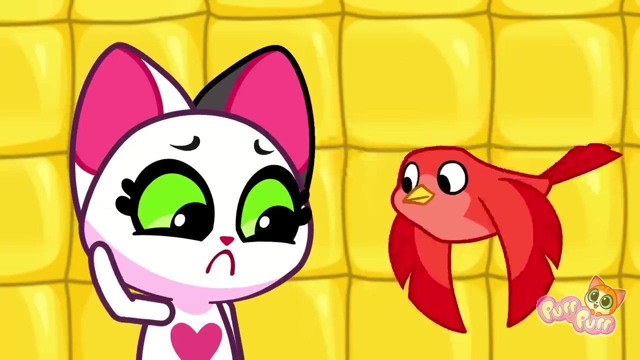 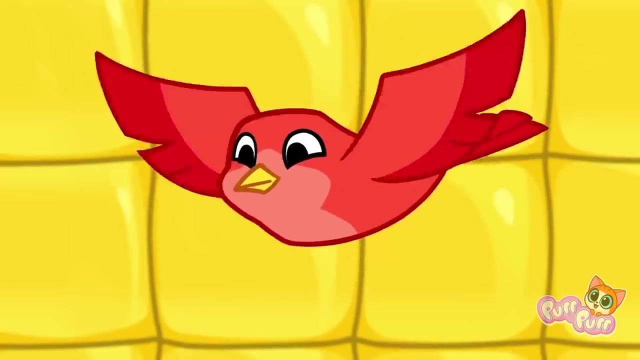 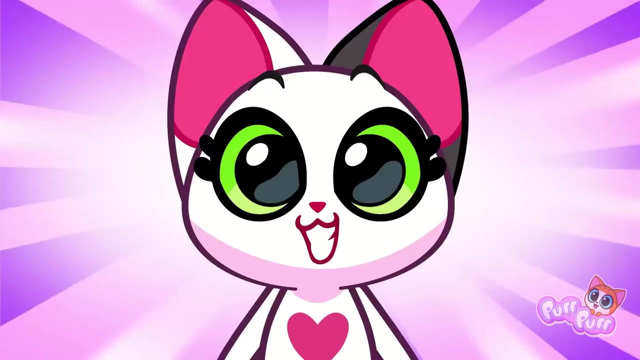 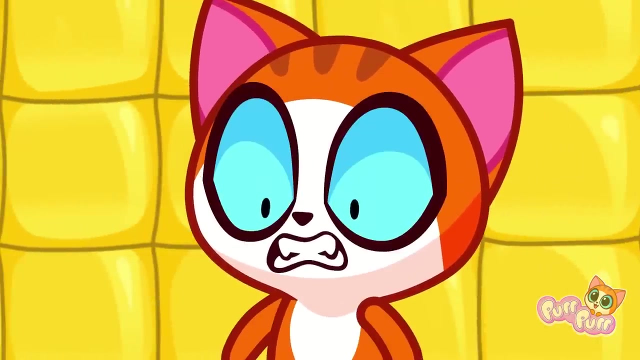 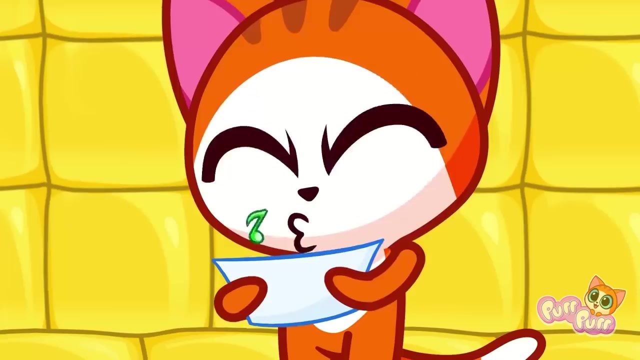 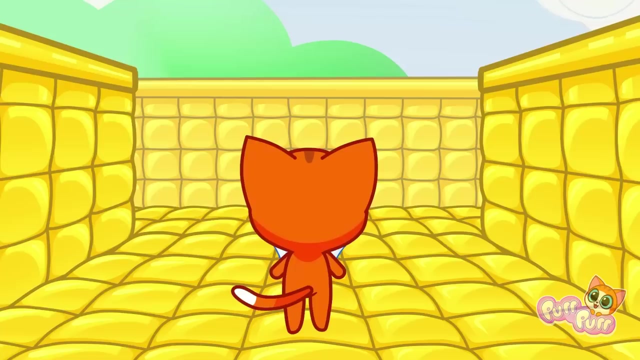 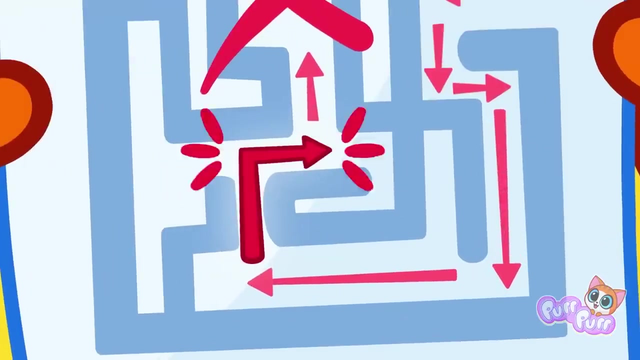 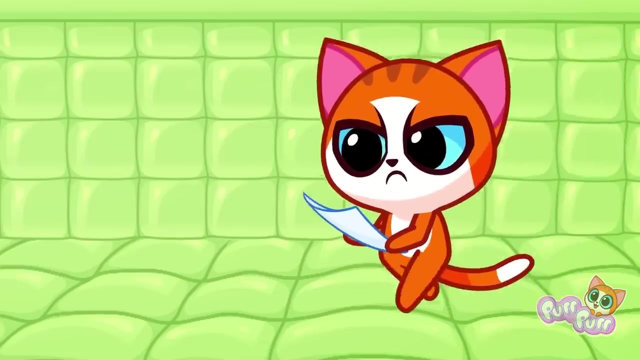 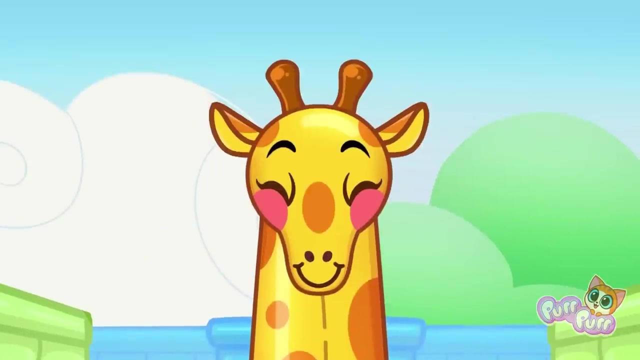 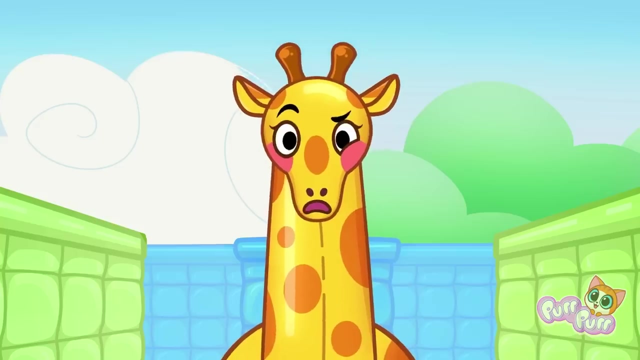 Let's eat. Do not disturb people around you. These slippers will save your feet. Please forgive us. Green Blue Red. Choose my favorite color. Green Blue Red. No, No, Rat No No.